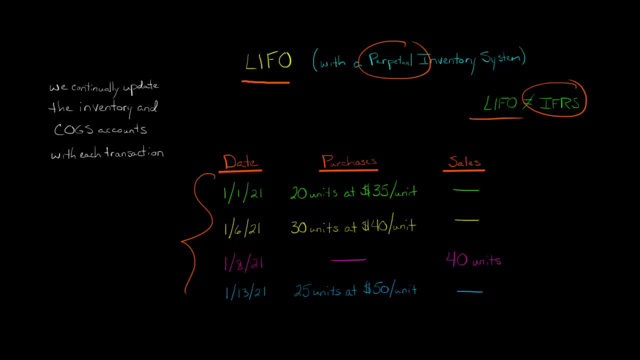 So let's say that we had a company with a series of purchases. so we've got a retail company. Let's say they make clothing for cats, So they make purchases of this cat clothing and then they sell some occasionally. So on January 1st they purchased 20 units at $35 a unit and then 5 days later they purchased 30 units for $40 a unit and then on January 8th they sold 40 units. 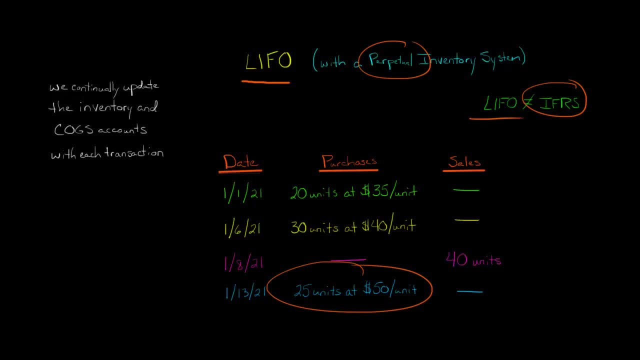 Now they also made a purchase later. but here's the thing: Because we're using a perpetual inventory system, we're going to continue. We're going to continuously update the inventory, but also, in some cases, when we make a sale, the cost of goods sold account whenever we have a transaction. 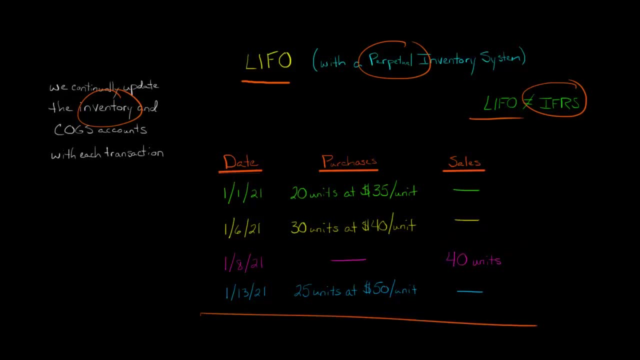 Periodic is different Periodic inventory system. we wait until the end of the period and then we say, okay, let's do our LIFO: last units in or the first out, the cost of goods sold and so forth. But here it's different When we're perpetually doing it, here's what's going to happen. 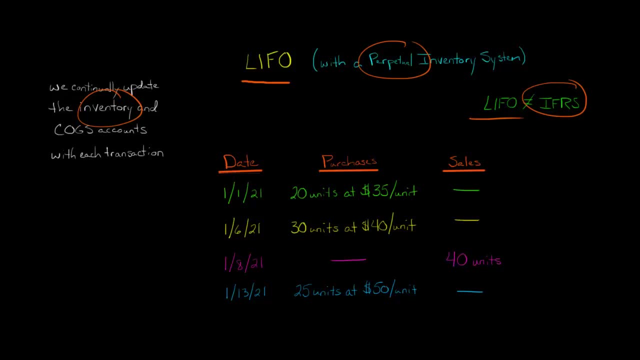 So on the 1st we're going to say, okay, well, we bought 20 units at $35 a unit, So we're going to increase inventory by $700, right? And then we're going to increase inventory when we make another purchase. 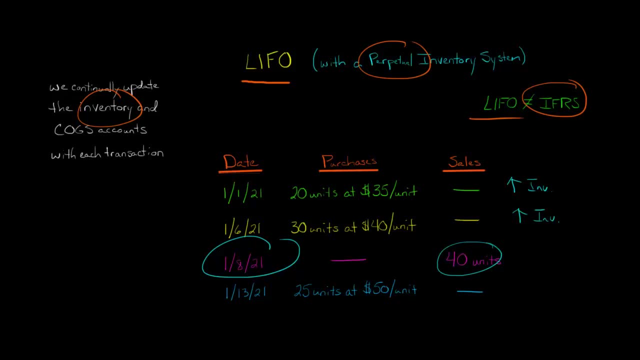 But then on January 8th we sell 40 units of inventory. So as of this point in time, January 8th, we have to make a journal entry. We have to make a journal entry and we're going to debit cost of goods sold and we're going to credit inventory. 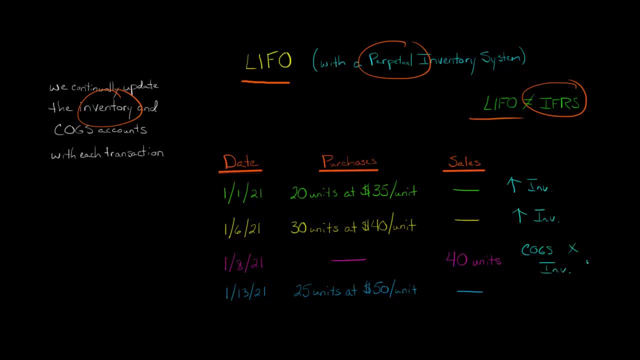 But the question is: how much? How much are we going to do this for? Because we have to use LIFO as this cost flow assumption to see what the numbers are here. okay, We don't wait until the end of the period to do it. That's periodic. 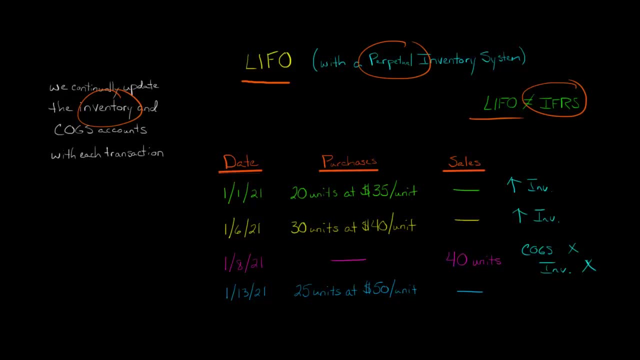 And we're going to do it as of right now. So think about it like this- I'm going to ignore this right here because, as of January 8th, we don't even know that this is going to happen yet- Like this is the future, January 13th is the future when we're talking about January 8th making this journal entry. okay. 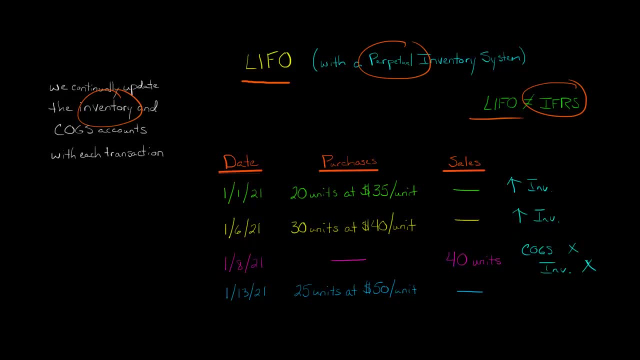 So that's going to be confusing. It's going to be confusing for some people. If it is, check out the video on LIFO with the periodic inventory system. But here we go. So we sold 40 units, okay. 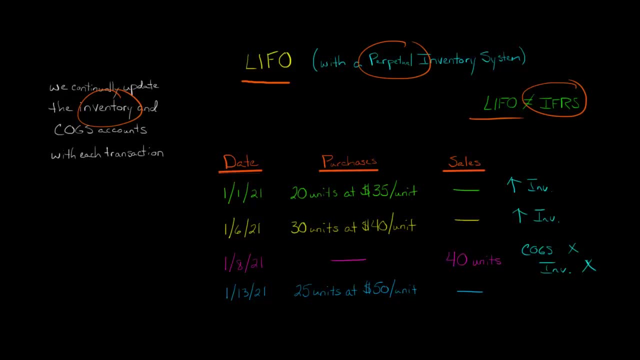 So on January 8th we're going to say: okay, LIFO is last in, first out, So of those 40 units, we're going to take the 30.. Those are the most recent purchases. Okay, so we're going to have 30 units at $40 a unit. 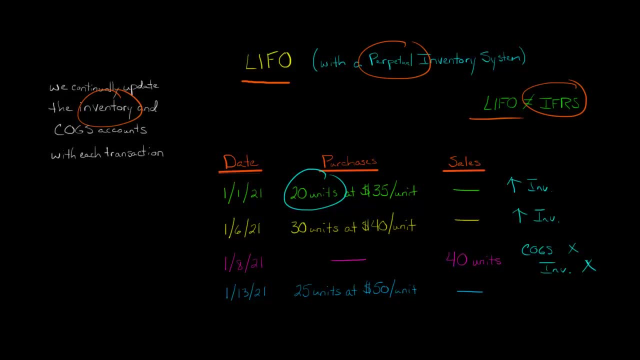 But then we have 40 sold, so 10 are going to come out of this right. So from January 1st we're going to have $40 a unit. So we're going to have $40 a unit. 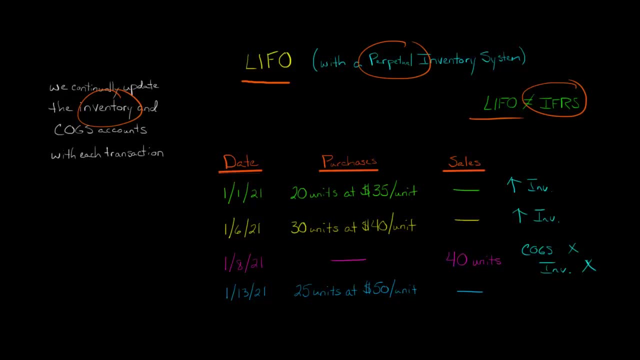 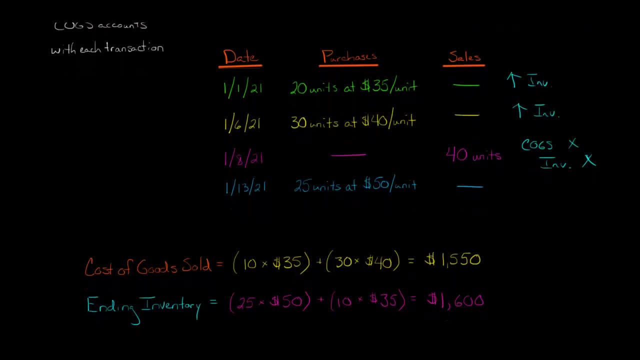 That is going to be the cost of goods sold, And then everything else, because this is the only sale that we have here. everything else, at the end of the period our ending inventory is going to be $1,600.. Let's say at the end of the month or whatever, assuming these are the only transactions, okay. 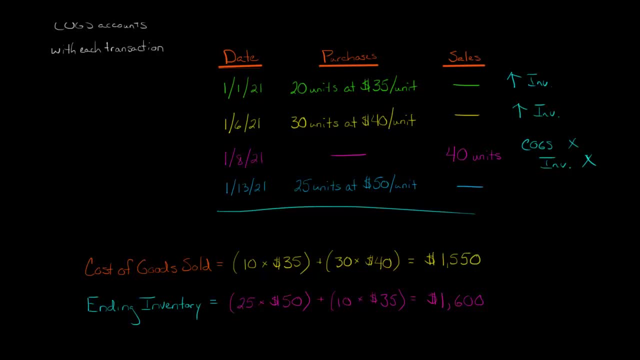 So in the ending inventory. so basically, so we took the $30 went to cost of goods sold, and then $10. And then of that $20 went to cost of goods sold. So then the ending inventory is going to include the remaining $10 here at $35 a unit. 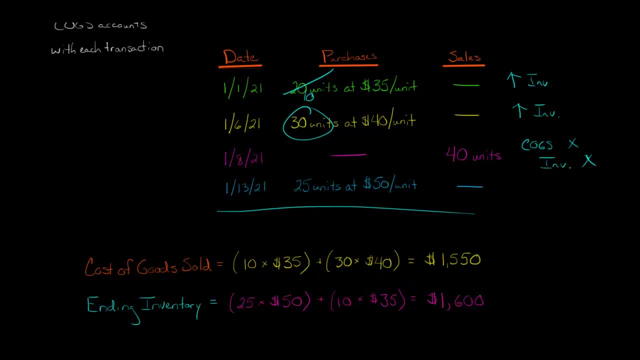 And then it's going to have this $25 at $50 a unit. okay, That's the end of the period. Let's say January 15th was the end of that reporting period, And so we say, okay, here's what the ending inventory is as of that time. 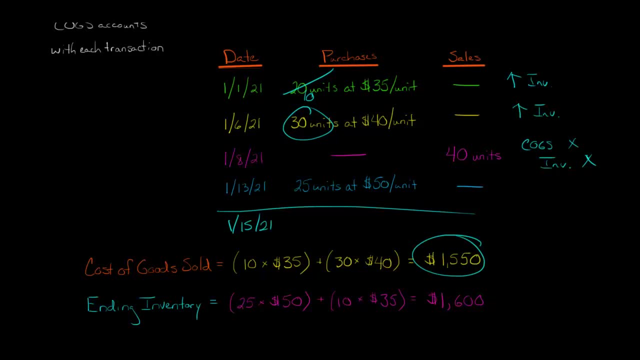 And then the cost of goods sold for that month or that two-week period, whatever it is, would be $1,530.. So the key is- and this is what confuses people when you're using LIFO with the perpetual inventory method- 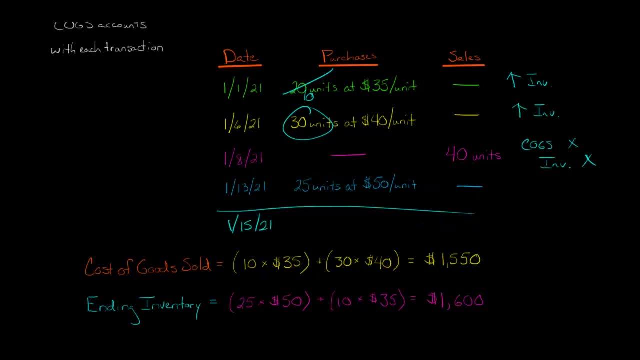 if you have some transaction here, remember that as of January 8th, this hasn't happened yet. okay, So perpetual. we're saying: okay, here we bought inventory. okay, let's increase the inventory account. Buy more inventory. let's increase the inventory account. 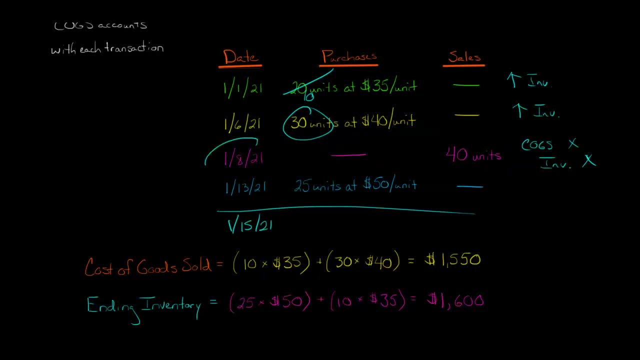 Sell inventory: okay, as of this date, January 8th. what are the most recent purchases? okay, The most recent purchases here was the $30, and then here are 10 of those $20,. okay, And that's how we figure the cost of goods sold. okay.